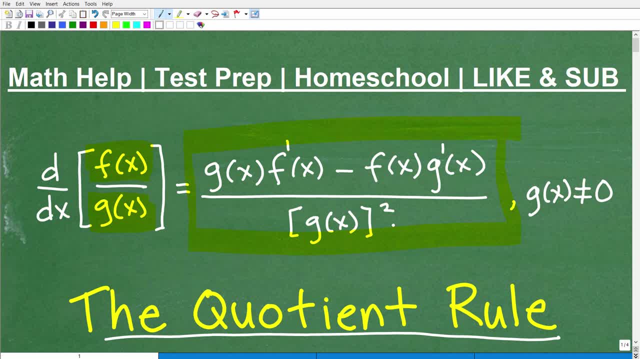 scary and whatnot. don't panic, you know, get what you can from it. But for those of you that are in fact taking calculus right now, well, this is kind of fundamental, foundational stuff that you absolutely need to know. So we're going to get to all this in just one second, But first let me quickly introduce myself. My name is John. I'm the founder of TC Math Academy. I'm also a middle and high school math teacher. I've been teaching math for decades And I'm telling you right now, if you're at the calculus level, you already know how to be successful in mathematics. you already realize. 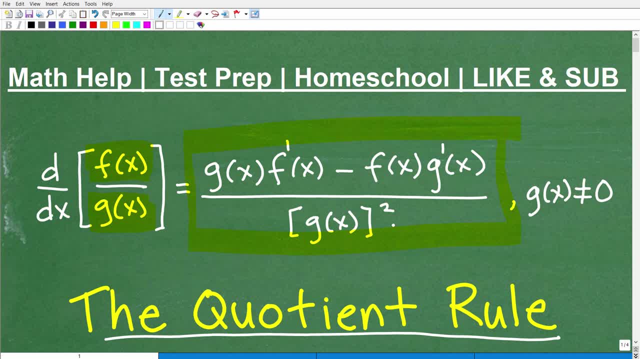 that it takes a lot of effort to learn math, But what you need beyond that is great math instruction. Hopefully you have a great professor teaching you calculus. I actually don't offer a calculus course. My highest course that I could offer you is pre calculus And a lot of people struggle in calculus because they haven't really mastered everything in pre calculus. So if you need assistance with kind of that foundational stuff- all the advanced trigonometry, polar equations- 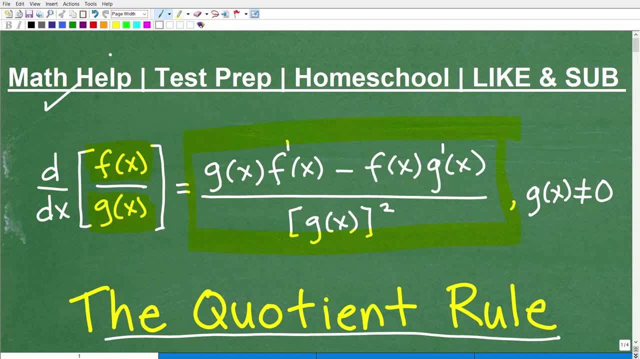 logarithmic functions, all that kind of stuff that you definitely need to know to be successful in calculus. check out my pre calculus course. you can find a link to it by going to my math help program. you can find a link to my math help program in the description of this video And then you can find my pre calculus course there. So if you're shaking on that kind of things that you should have learned in pre calculus so you still don't know, well, that's going to show up and have a negative impact on your math. 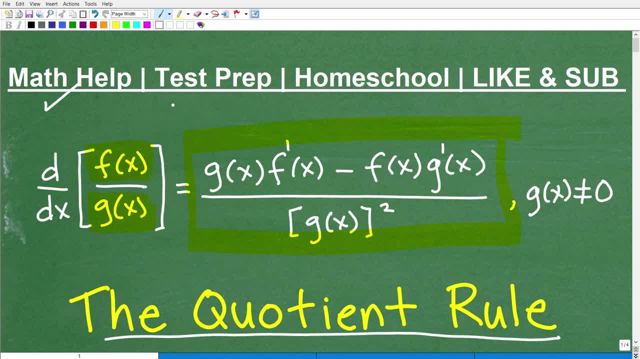 on your study, your calculus studies. So, anyways, that's one thing I can offer you. Also, if you're preparing for any sort of test with a math section, like a teacher certification exam, ASVAB, GRE, GMAT, etc. I have a ton of test prep courses that can help you out. If you happen to be homeschooling- you're just checking this video out- I have a ton of middle and high school courses for homeschoolers, So that's something that, if you are interested in, you could check out. And if this video helps you out, don't forget to like and subscribe. 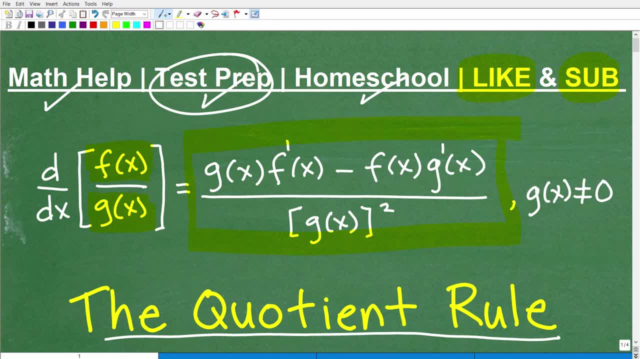 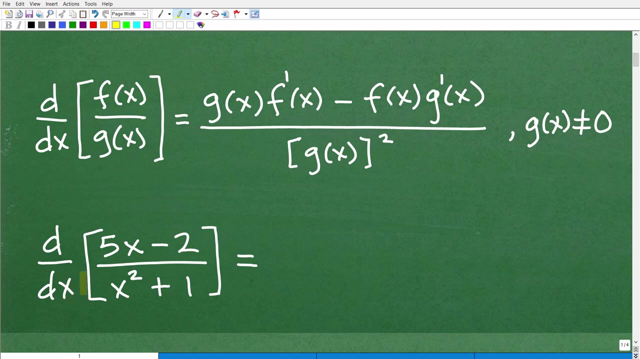 That definitely helps me out. So, again, I don't know where you're coming from. Some of you out there might just be watching this video just because you're interested in calculus, And that is awesome as well. But let's go ahead and get into the quotient rule. This is definitely basic calculus. you absolutely need to understand this. And let's go ahead and see how this works by looking at it. an actual example. Okay, so let's say I want to define the first derivative of this function right here. 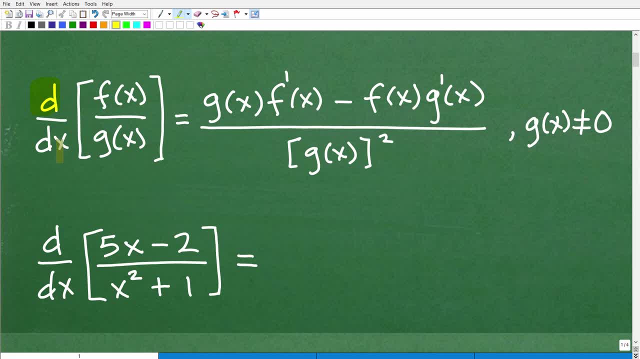 This expression: okay. now this is finding d of dx, okay, which is basically the first derivative. So this is the notation. there's other notations. you can use the prime notation, like y finding y prime. So that's you know other notation that you might be familiar with. But here what I'm saying is go ahead and find the first derivative with respect to the variable x of this function, right here. Now, if you look at this function, you could see 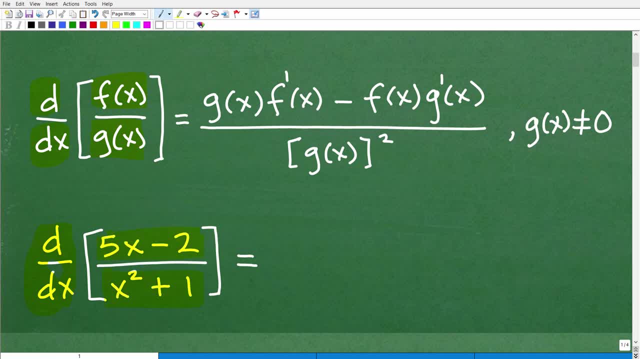 we have a numerator and a denominator. Technically this would be classified as a rational function. But you know, you look at it, it's like, hey, it's or there's a fraction going on here. right, There's a numerator and denominator, So how can I find the first derivative of a situation like this? Well, this is a quotient. Okay, remember the word quotient has to do with division or fraction. So anytime you see something like this, where there's a fraction going on, you want to be thinking. 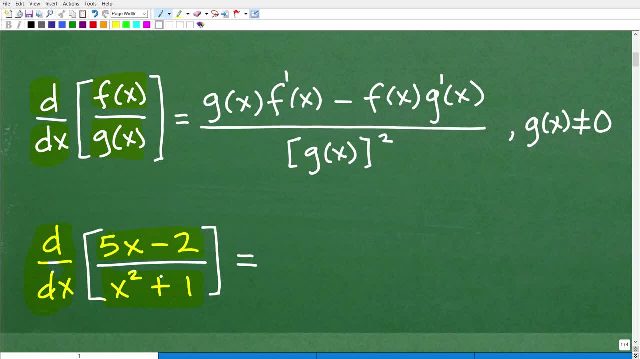 quotient. Okay, there's other rules, like the product rule, etc. But so, anyways, we are going to apply the quotient rule And here it is Okay. so let's just kind of look at the quotient rule And what does it say? Well, here we have a numerator And here we have a denominator. So the denominator starts off by saying: you're going to take that g of x function, which is the function that represents the, or the function in the denominator. In this case it's going to be x squared. 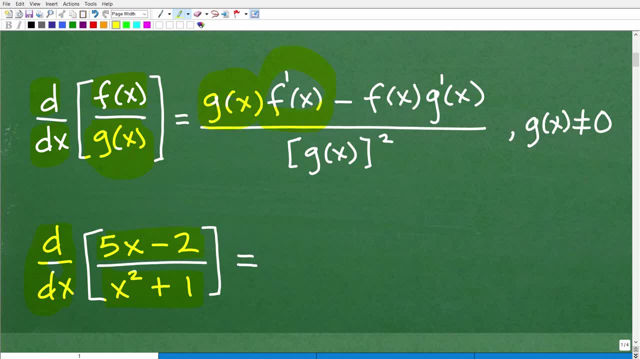 Plus one. So you're just going to write that And you're going to multiply it by the first derivative of the function in the numerator. In this case, that's five x minus two. Okay, so yes, you're going to have to use a lot of algebra to kind of set all this up, But this again, it's not difficult. Now, hopefully you already know how to find the first derivative of these little functions right here. If not, I'll show you exactly how to do that. And then you're going to put a subtraction sign And then we're 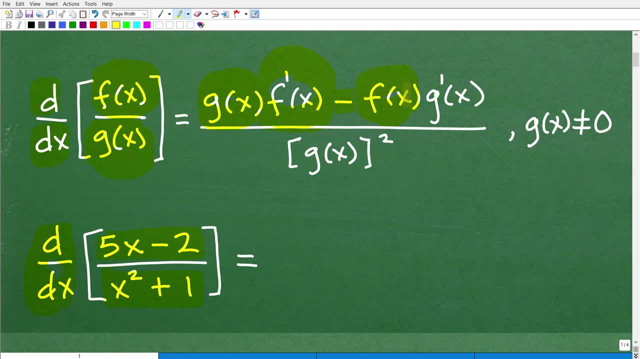 going to put the f of x function, which is the function in the numerator, right here. we're going to multiply it by the first derivative of the denominator function, which is x, squared plus one. That's what this is. So this is a lot of math. That's our numerator. So we're going to put a nice long fraction bar right here And then we're going to put that all over the g of x function, which is our denominator function, squared. Okay. so when you're looking at these rules, 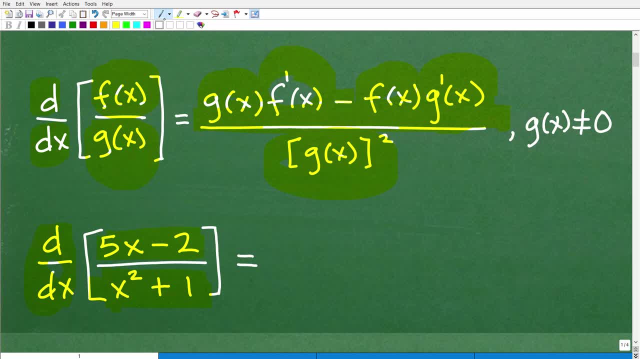 you know, obviously you know. before you commit this to your memory- and this is something you probably would not be given on a test or quiz in your calculus course- you probably your teacher is probably going to ask you to just do problems without like a little formula sheet. it might give you a formula sheet for your final exam, But some of the stuff you definitely want to commit to long term memory And there's other notation that you can use. that's a little bit easier than this, But anyways, I would just want to kind of break. 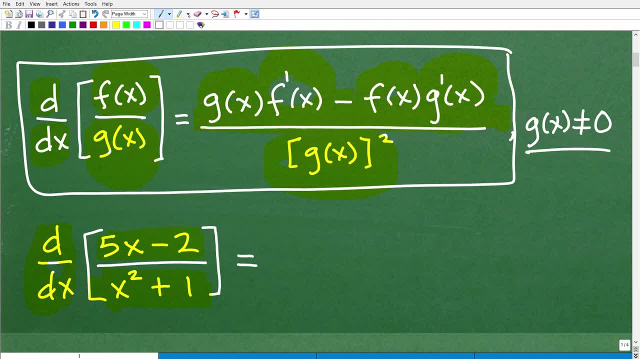 this out. This is the quotient rule, And you can see here that the g of x function cannot be equal to zero, because we don't want to have zero in the denominator. Okay, so if you are, you know, at the pre calculus level or calculus level, or you have some, you know, pretty decent math skills, go ahead and set this up. Okay, follow this rule Again, right here, this top function, this is the f of x function and our 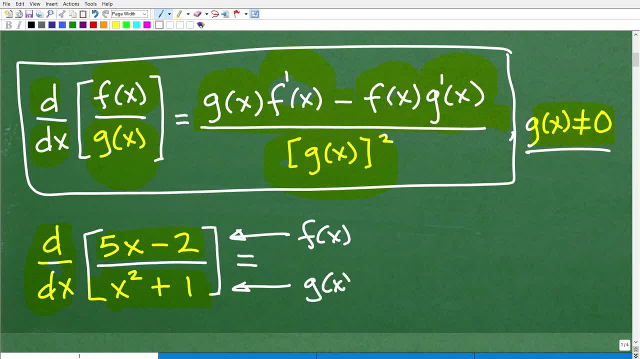 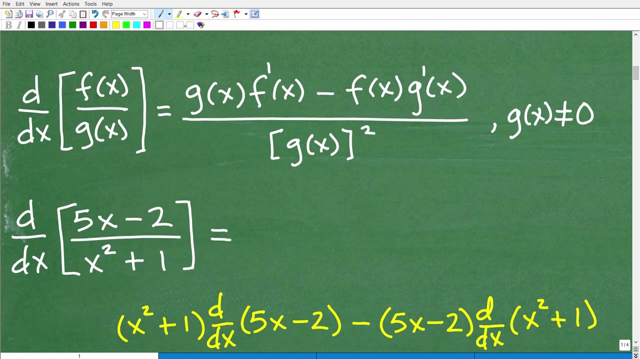 bottom function down here in denominator. this is our g of x function, And all you got to do is kind of set this up by following the rules And then this working this down. Okay, so let's see how well you can do with this. I'm actually going to show you the answer. If you're not ready to see the answer, go and pause the video, But I'm going to go ahead and do this right now. Okay, so here is the quotient rule. Okay, here is our problem. We want to find the first derivative with respect to 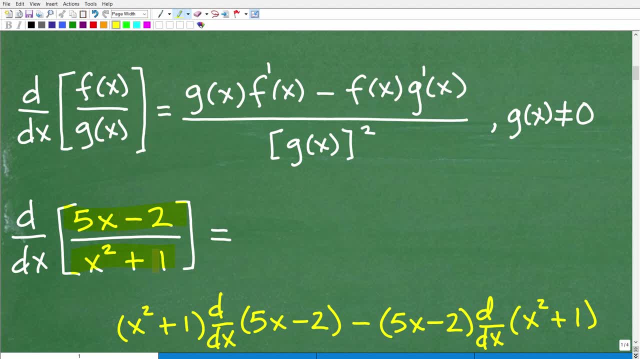 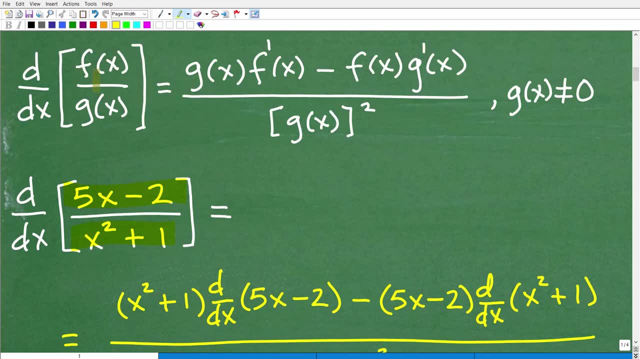 x, 5x minus two over x squared plus one. So let's go ahead and write this out. Okay, now I'll kind of shift back and forth. So we're going to say, Alright, so here is the quotient rule. So we're going to first start off by writing that g of x function. Okay, this is again notice. the g of x function is the function in the denominator. So we're just going to write that out And I have that right here: x squared plus one, And we're going to multiply it by 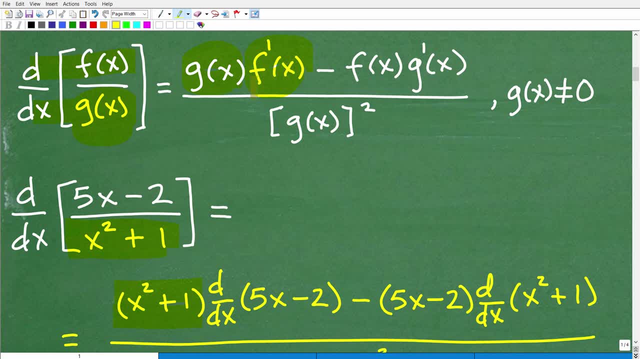 f, prime of x. this is the first derivative of the function in the numerator, So this is 5x minus two. So I'll use this notation right here. Okay, we're going to take the first derivative, with respect to x, of 5x minus two. So that's what this is right here. Okay, this is the first derivative of that numerator function, which is, of course, 5x minus two. Okay, now we're going to put a subtraction sign, So I'll write that there. Then I'm going to put what? 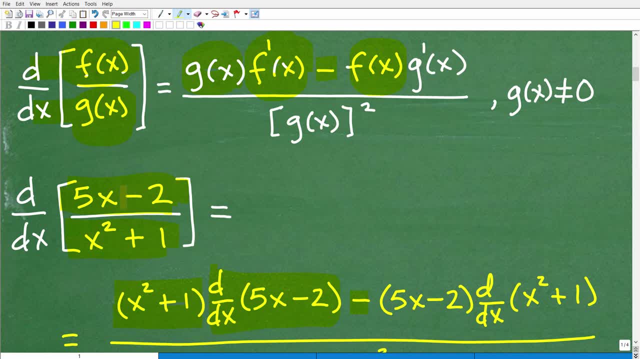 I'm going to put f of x, which is the numerator function, which is 5x minus two. put that there. And then we're going to put the first derivative, with respect to x, of that g of x function. That's our denominator function, x squared plus one. So we'll write that right here. This means find the first derivative, with respect to x, of that denominator function, x squared plus one, all over g of x squared. Okay, so let's put that right here. 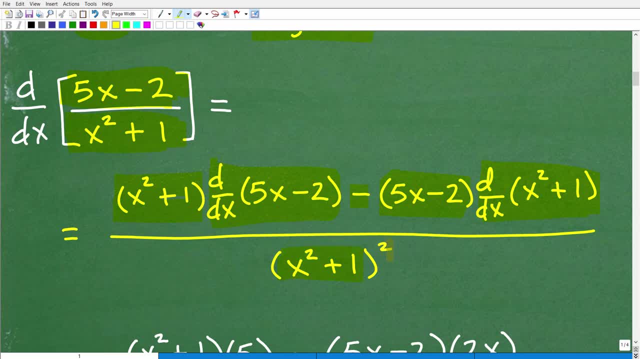 g of x squared again, is that denominator function? And then we'll square it. Okay, so this is the setup, And anytime you're working with any formulas in calculus or mathematics, before you start doing the work, you want to double check. hey, did I do this right? Okay, yes, here is the g of x function. This is the first derivative of the f function minus the f function times, the first derivative of the g function. And here is the g function squared. 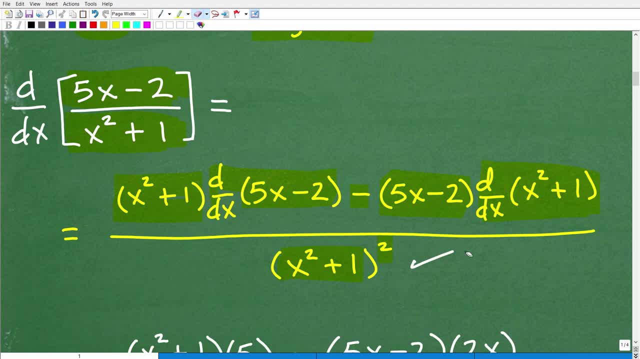 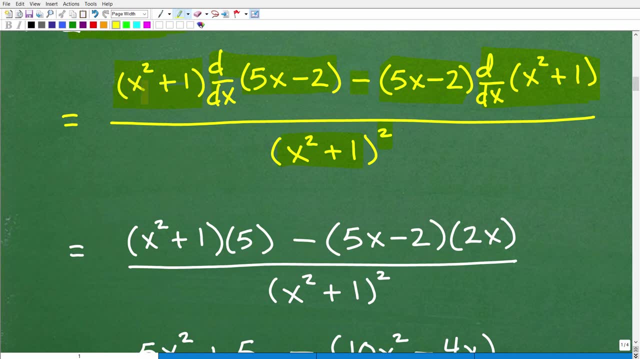 Okay, so you're going to look at all of that and you're like, okay, that makes sense. So now let's go ahead and actually do the work. Okay, so let's start off here: x squared plus one, So that's just going to be x plus one times the first derivative. I'm focusing on this part right here of 5x minus two. Okay, so what's the first derivative of that? Well, let's kind of do this right here: 5x minus two. If I'm taking the first derivative, are you going to? 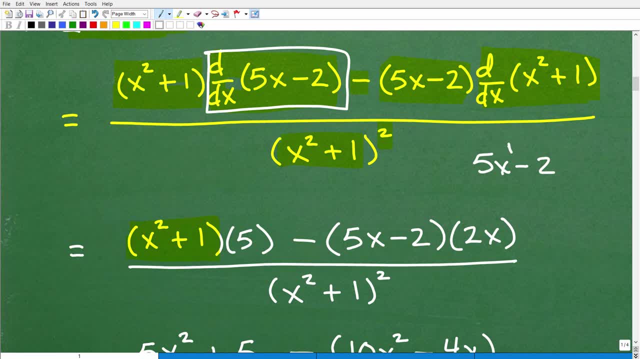 do is the power rule right? So there is a one right here. it's going to multiply that one times that five, So that's five times, and they're going to drop this down as this is going to become x to the zero power, So this is just going to be equal to five. Now, if you don't know how I got five as the first derivative, then you want to look at other videos using a power rule, the chain rule, all that kind of good stuff, basic calculus, Okay, how to 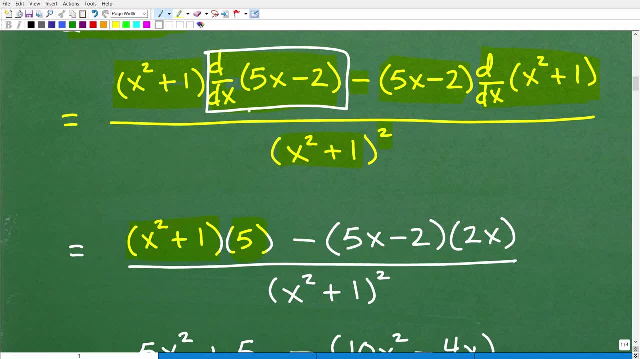 find the first derivative. So you do need to know some of that basic stuff in order to use the quotient rule. But anyways, here is our first part of this problem. So now let's go ahead and work on the second part. So here we have 5x minus two, So we'll just write that there, And then the first derivative of x squared plus one. Again, I'm going to take this x squared plus one. take this two multiplied by the coefficient, that's going to be two times x, and drop that power down by one, So that'll be two x. 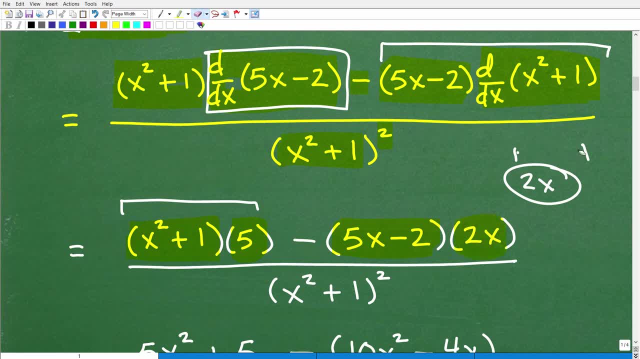 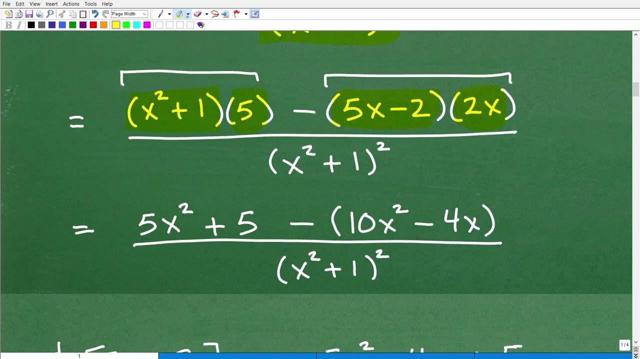 Okay, All right. So that's how you find the first derivative of these nice basic functions like this. And then here this is going to be x squared plus one squared, And we will just leave this expression in its current form. we won't actually do all this multiplication, It's not necessary, But anyways, now let's go ahead and clean this up. Okay, All right. So here we have 2x times 5x minus two, So I'll just use the distributive property. take two. 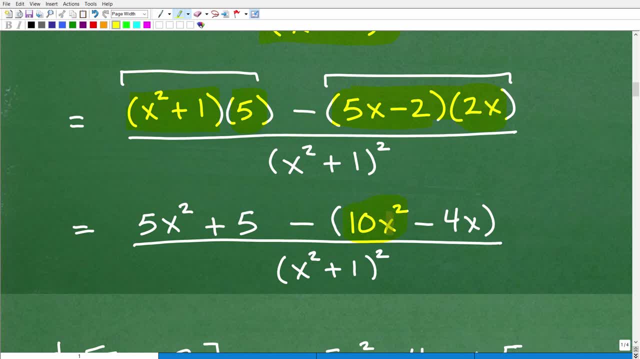 x times 5x, that'll give me 10x squared. and then 2x times this negative two, that'll be minus 4x. So this is all going to be in parentheses because I have a subtraction sign here. you got to be very careful. A lot of people get in trouble with the quotient rule because they mess up with their algebra. And then here I have five times this x squared, that gives me 5x squared. five times this one is five. So now we're just going to be 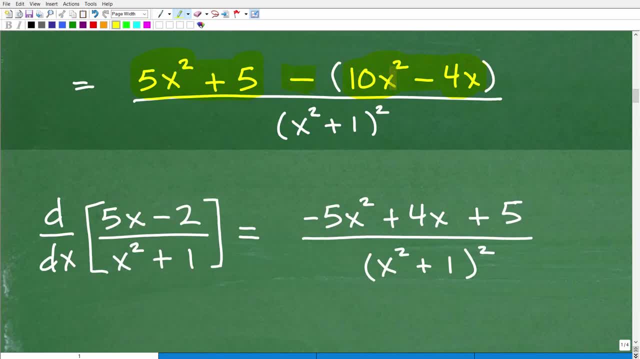 very careful with our negative sign. So this is going to be negative 10x squared, And I have two like terms here: 5x squared and negative 5x squared, or sorry, positive 5x squared minus 10x squared. excuse me, when I distribute this negative, when I combine these like terms, I end up with negative 5x squared. then this negative okay times this negative 4x is going to be a positive 4x, And then that leaves me with a positive five up here in the numerator. Just go ahead and leave my 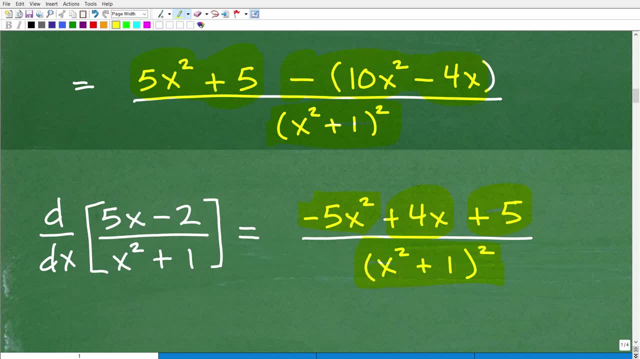 denominator, like so x squared plus one squared, And there you go. Okay, here is the first derivative of this rational function. Okay, And we use the quotient rule. Okay, again we're seeing we got division going on here. we have a numerator and denominator and we just kind of simply follow. 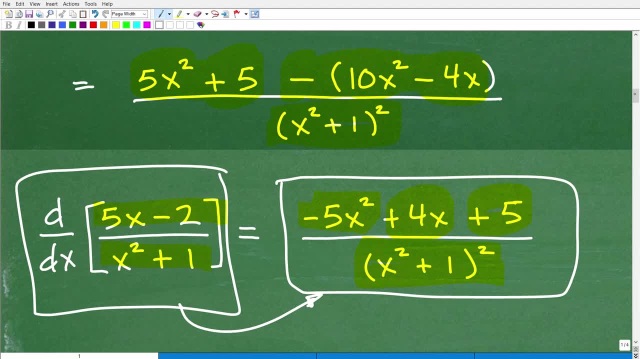 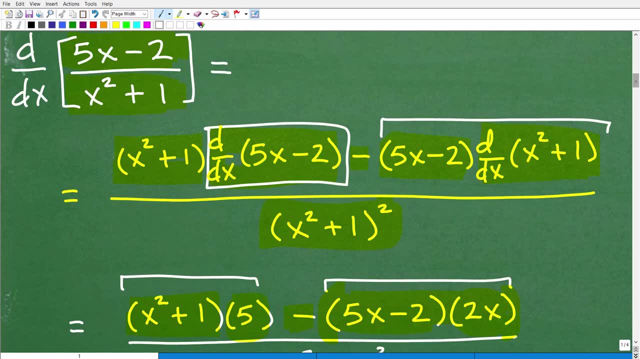 the rule, But we have to be very careful with the algebra. Okay, And of course, you also need to find, or know how to find, the first derivative of these nice basic functions. here Again, if you're looking at this video and you're like, oh yeah, the quotient rule, I'm studying it all this other.